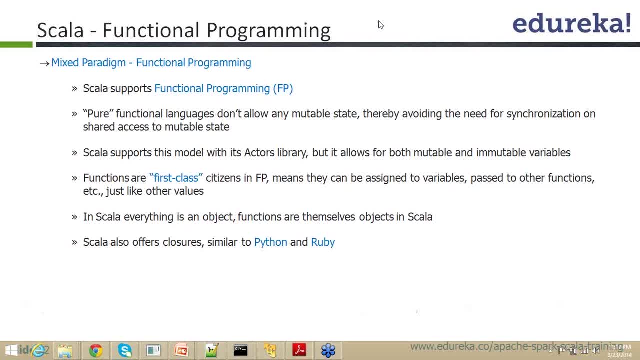 not VARs. Now, VALs and VARs are some of the new things which are coming to you without even informing what they are It's all about. typically they say: work in the terms of constants, don't typically work in the terms of variables, So we will talk about that. So, typically, this: 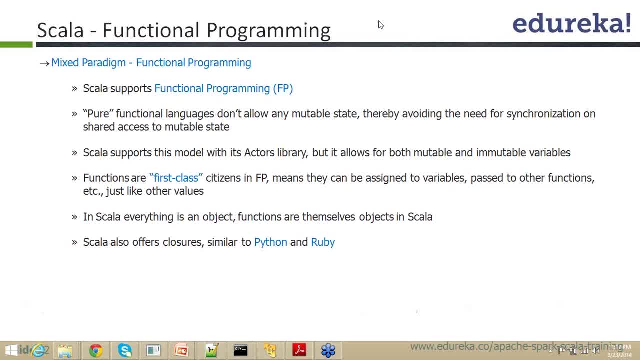 is the way Scala works, In fact it's. unless you really require it, you should not even create the VARs in Scala. So you'll see that It is typically very, very, I would say, native to a functional programming style rather than the object oriented programming style. By the way, I do understand that many 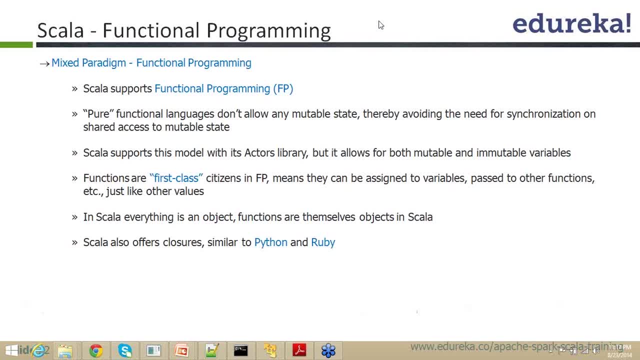 of you might have worked on the Java, might have have already worked in Java environment, So you must be very, very good from the object oriented side. Very good, Keep it with you. But before we start on, let's say module number four. right, 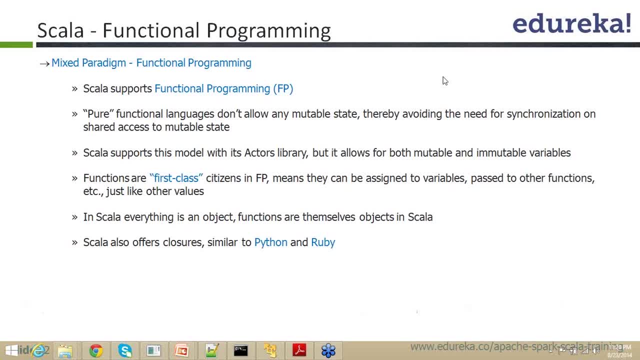 it would be really good if you can just take a very quick refresher of functional programming. You can just take a very quick kind of an idea about it. It really helps nothing else. Functions of the first class regions: I think I have just told about it. So they are actually. 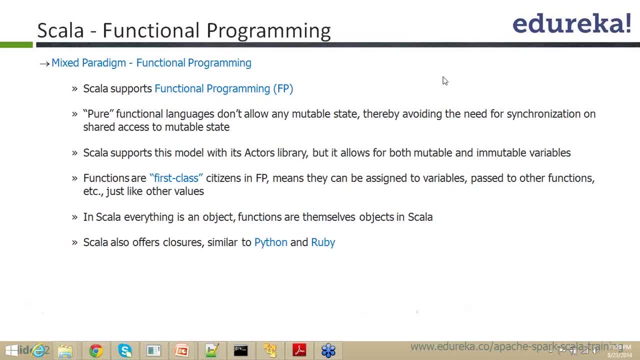 treated just like variables. The way you treat variables, you know. you can pass them to the functions. You can pass a function to the other function. You can write another function within a function. Okay, A lot of other things, right, So we'll. we'll come to that part in details whenever. 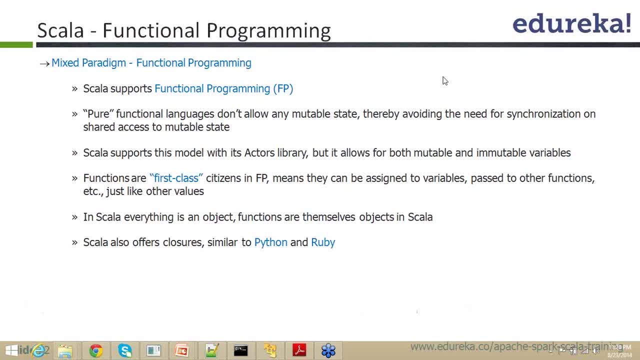 you know we'll be visiting- about the function programming aspects of it, And also Scala offers closeness. Now, this is something you must have heard about lambdas right, Especially those people who are aware of Java 8, they have actually copied it. Okay, They have copied. 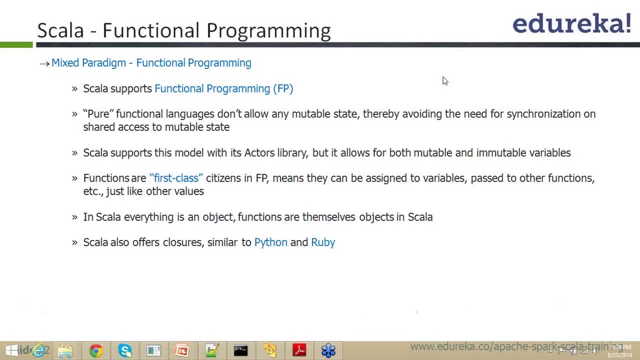 it. They copied it from Scala, Ruby Python, all that, Okay, Lambdas and all. So they are kind of, you know, you're so if, if I have to say, I'll just summarize it in a way that: 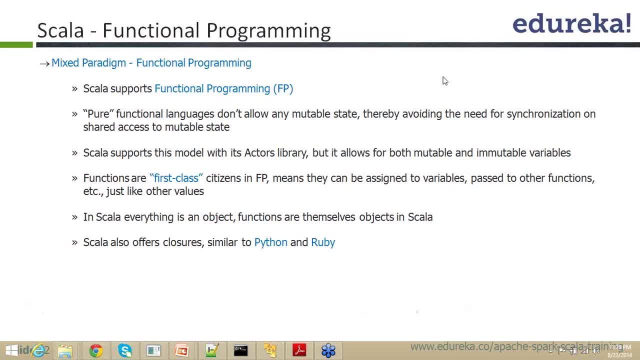 you know functions and all right, PL, SQL and all or any other programming language non-object oriented, because functions are not a word in object oriented world. right, In object oriented world, what is the equivalent of function? I mean, there is no word called. 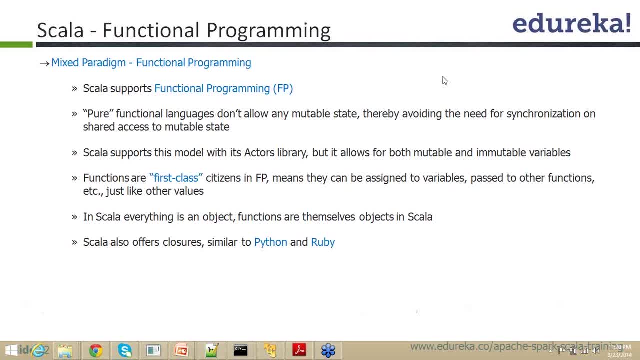 function. right, It is called method, And methods are typically associated with a class. and then you instanti, sheet a object and then you keep on calling, You pass the parameters to these methods which are invoked on those object instances. right, Guys? making some sense, right? So there is nothing called. There is nothing called a. 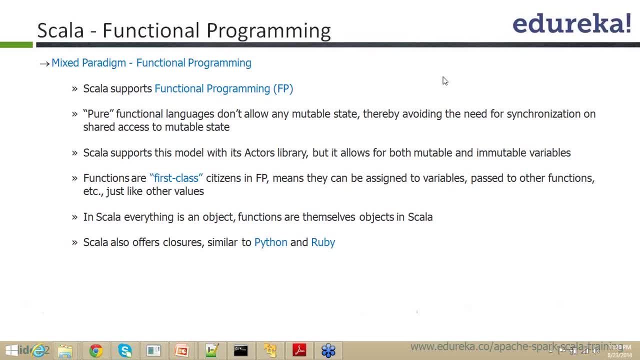 function. but here in this functional programming world- P, L, SQL, T and R- you must have heard. you must have heard about functions, procedures, packages. right, they carry a very different meaning than the methods of object oriented programming and the other. so the thing which 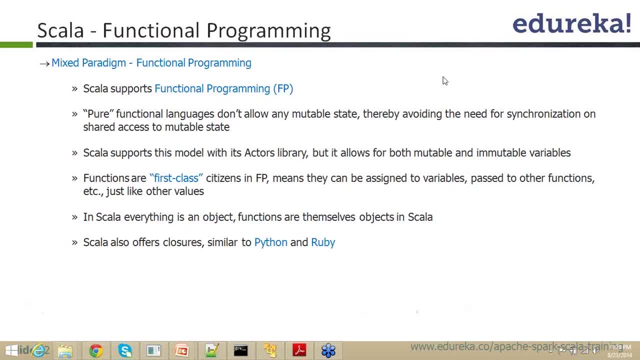 keeps Scala completely different from the other functional programming languages is that typically functions are named: function, calculate, radius, function, something right. so there are functions with some names and then their body. you can create anonymous functions in Scala: no name, just body. another different thing, right? but if you are coming from ruby, 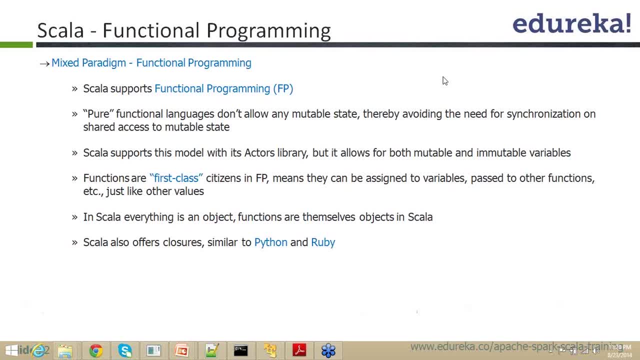 background or python background. it must not be new for you. so it is an anonymous function. it doesn't know. you just pass it to pass something to it. it will just work. it has no name, right in a different, convoluted way, we typically call them as closers. also, you will see that. 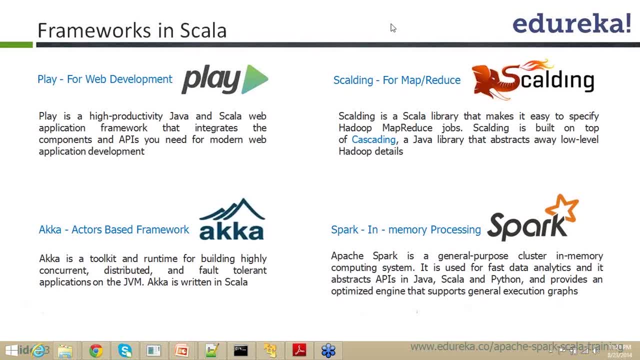 in quite a lot of cases, see this. so Scala is something which you are not really learning for. spark, by the way, just to tell you, akka, I have told scalding MapReduce. it's a framework which allows you to write your MapReduce jobs very, very fast. if you people are, if some of